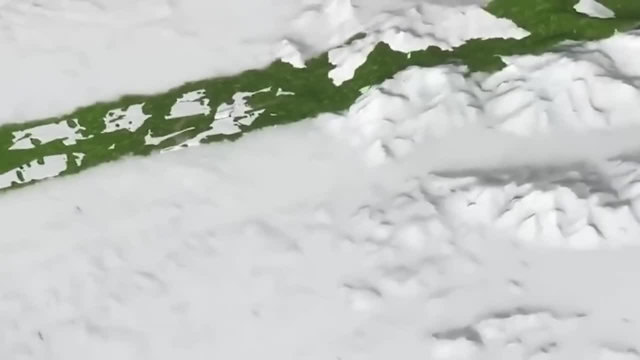 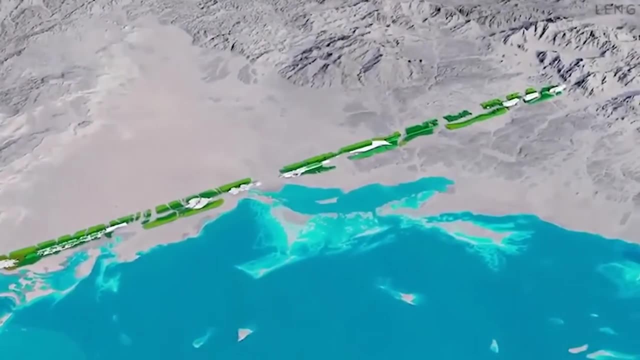 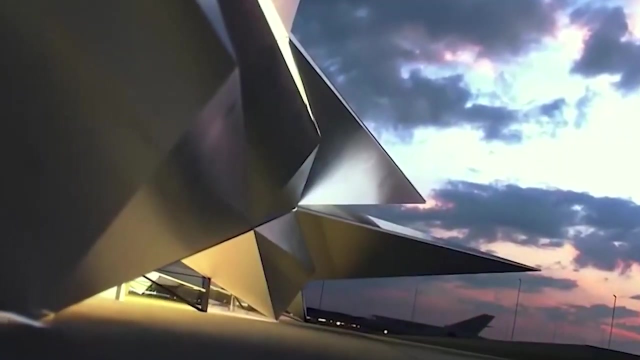 but that's just the tip of the iceberg. Without wasting time, let's directly get into the mind-blowing projects that are almost redefining human achievement and might leave you breathless. Number 10. Amala. Amala is a luxurious and exclusive travel destination in Saudi Arabia. dedicated to ultra-luxury wellness travel. It is situated along the country's northwestern coast and is owned by the Public Investment Fund, which is a key contributor to Vision 2030.. Amala is set to open its doors in 2028,. 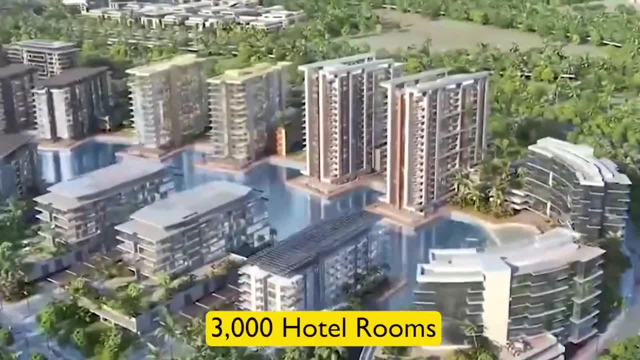 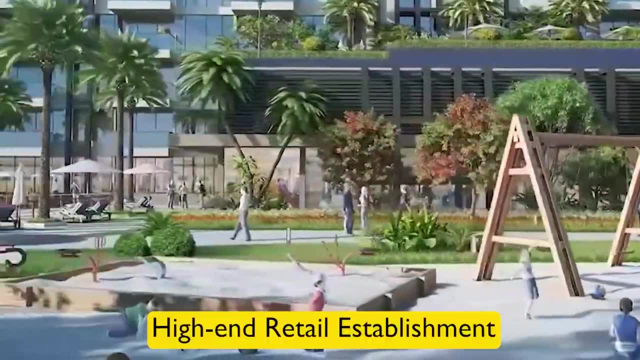 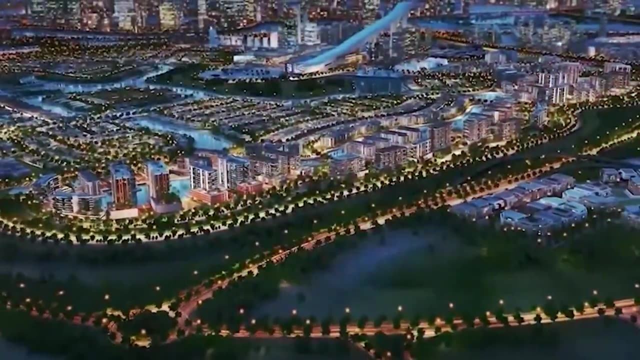 offering a range of amenities that include 3,000 hotel rooms, private villas, upscale apartments and estate homes. Additionally, there will be high-end retail establishments, fine dining options and state-of-the-art wellness and recreation facilities. The year-round destination is over 4,155 square kilometers. 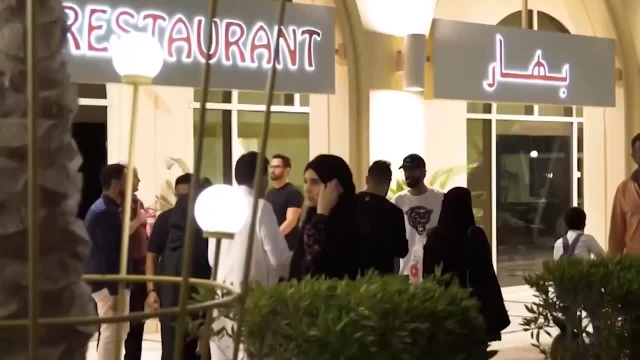 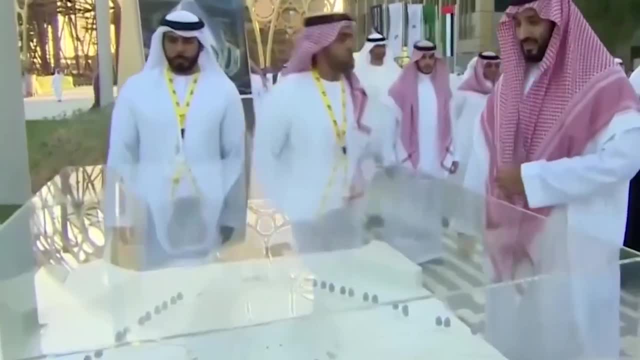 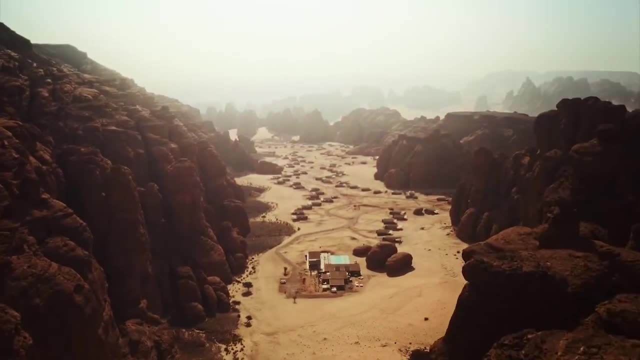 providing new tourism, wellness and cultural experiences for locals and visitors. Amala is designed to showcase the kingdom's strengths and create a more sustainable economy in the future. Number 9. Al Hula. Al Hula is located in the northwest part of Saudi Arabia. 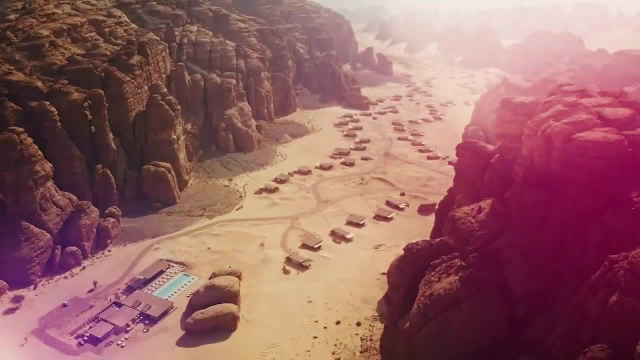 that is being made into a tourist spot. It has important historical and cultural sites, including the Old City of Agra, which became part of the UNESCO World Heritage List in 2008.. The area has beautiful natural scenery, like mountains, oases and interesting rocks. 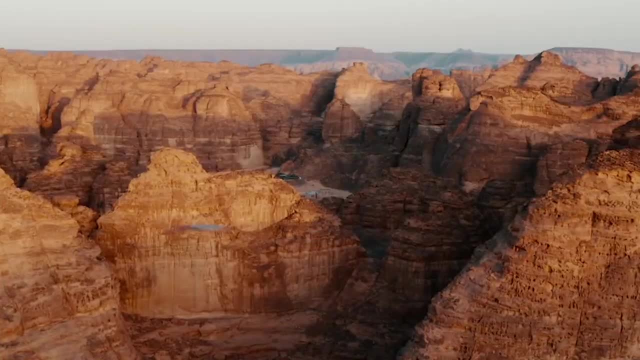 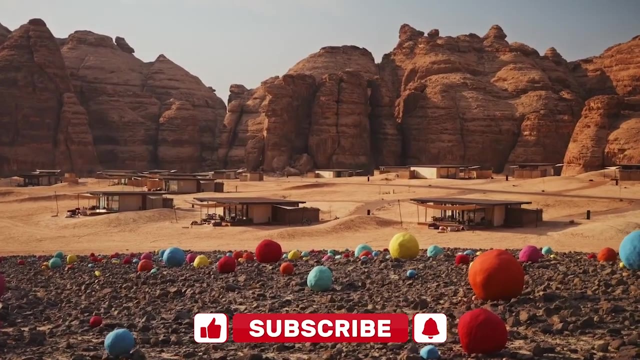 There are also traditional buildings and a lot of history. The Saudi government has invested much money to fix and improve the area so more people can visit. The project aims to create jobs for the local people and give tourists a chance to explore the area. The Al Hula. Al Hula is located in the northwest part of Saudi Arabia. 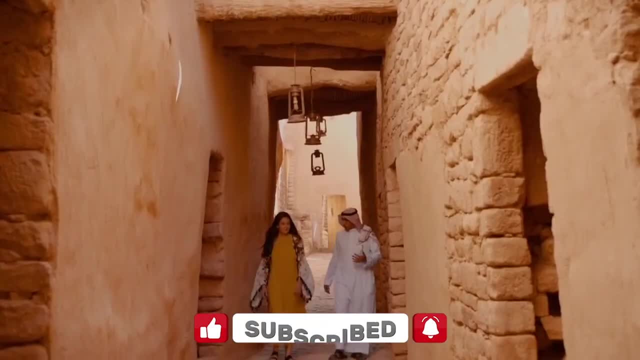 that is being made into a tourist spot. It has important historical and cultural sites, including the Old City of Agra, which became part of the UNESCO World Heritage List in 2008.. The area has beautiful natural scenery, like mountains, oases and interesting rocks. 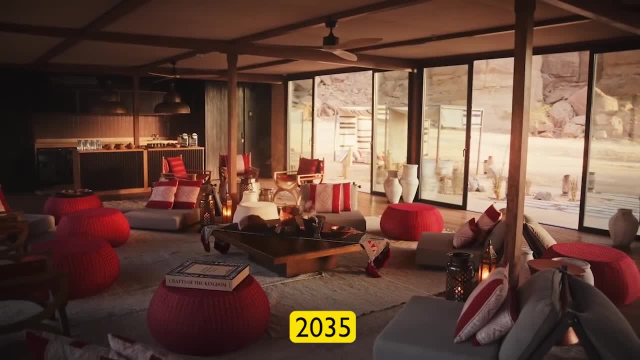 The area has beautiful natural scenery like mountains, oases and interesting rocks. By 2035, Al Hula should become a big attraction for people worldwide. By 2035, Al Hula should become a big attraction for people worldwide. This will help Saudi Arabia's plan to have a more diverse economy. 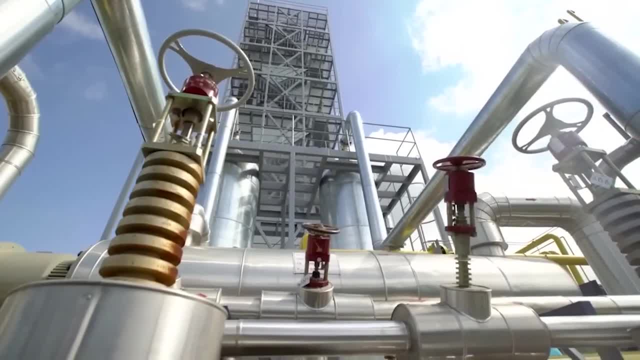 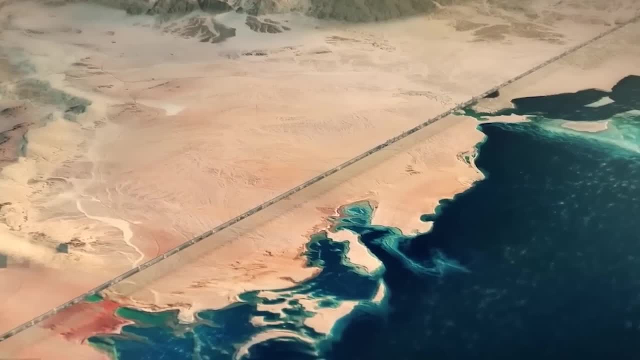 This will help Saudi Arabia's plan to have a more diverse economy that doesn't only rely on oil. Number 8, Newm. Newm is a planned cross-border city in northwestern Saudi Arabia. Newm is a planned cross-border city in northwestern Saudi Arabia. 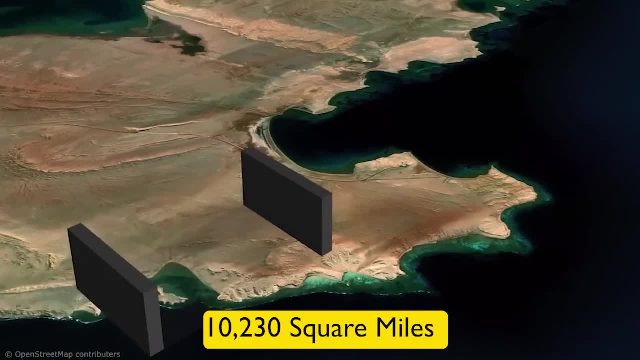 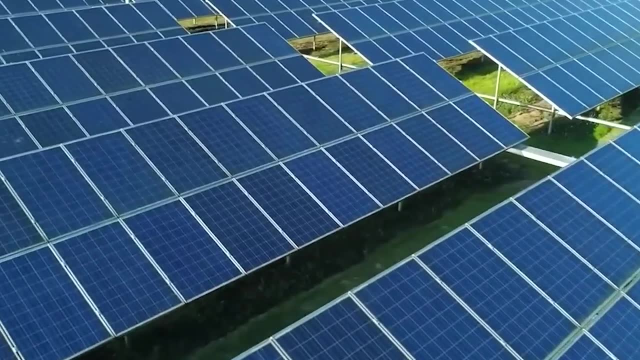 covering an area of 10,230 m2. covering an area of 10,230 m2 and is expected to cost 500 billion dollars. and is expected to cost 500 billion dollars. this project will focus on technology and renewable energy. The city's population will be over 1 million people. 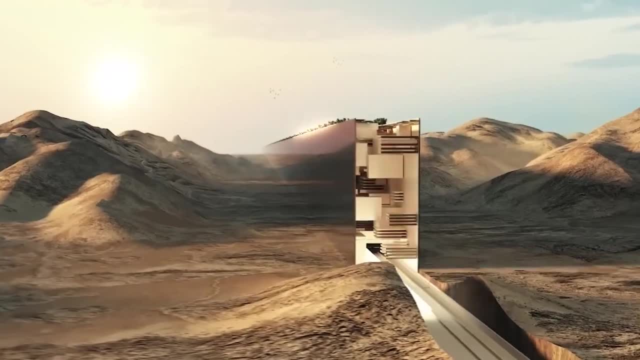 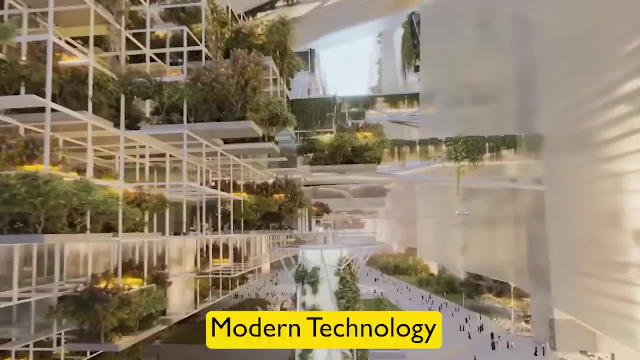 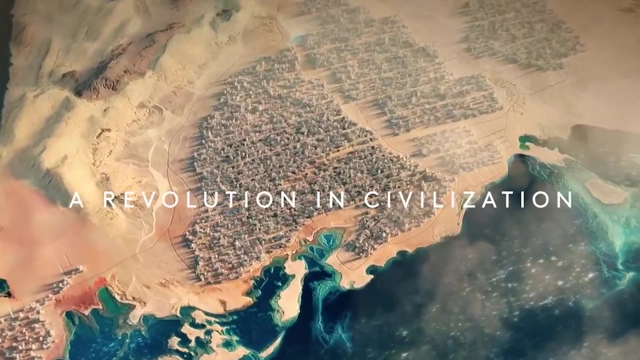 and it includes four different SUP projects. The four flagship projects are: a 105 mile long zero carbon urban belt, powered by renewable energy and modern technology. Sindala, a luxury island destination in the Red Sea that will be the first physical showcase of Neom. 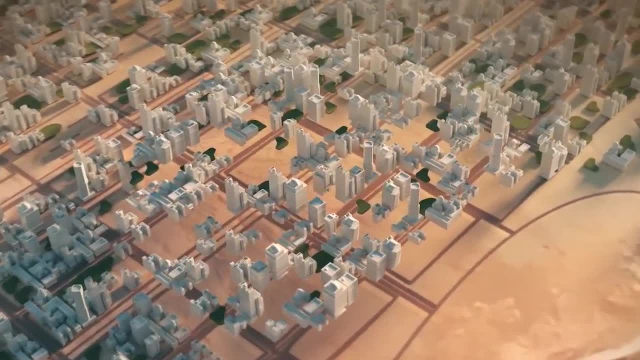 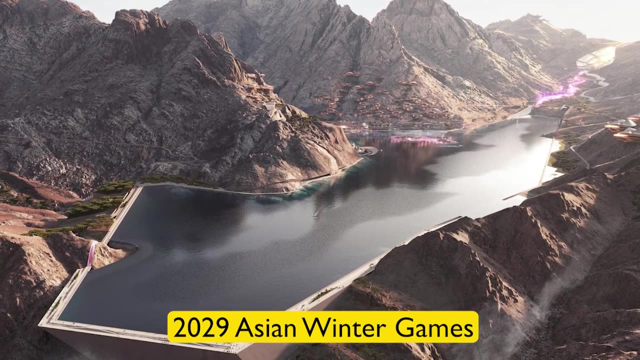 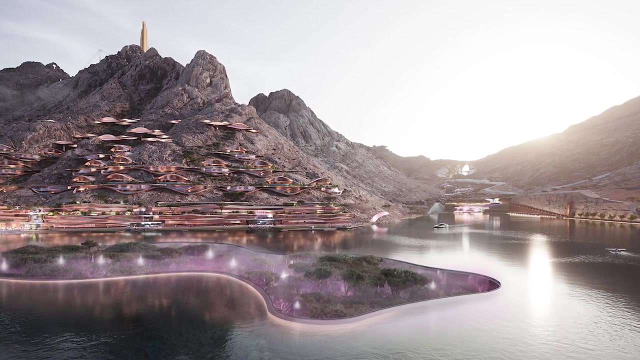 catering to the global yachting community and visitors seeking luxury. Trojana, a year-round mountainous destination. in Neom, hosting the 2029 Asian Winter Games. It will blend natural and developed landscapes to offer unique human-centric experiences for residents and visitors alike. And finally, Aksagom, a city where people 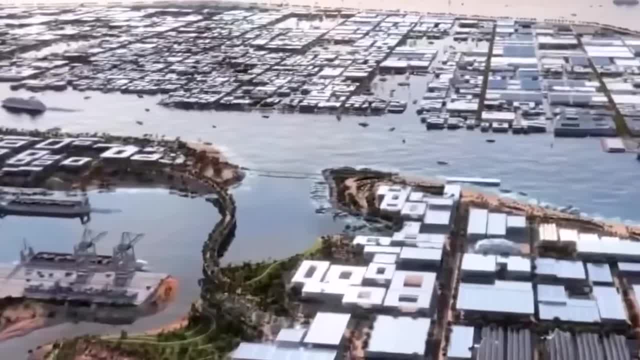 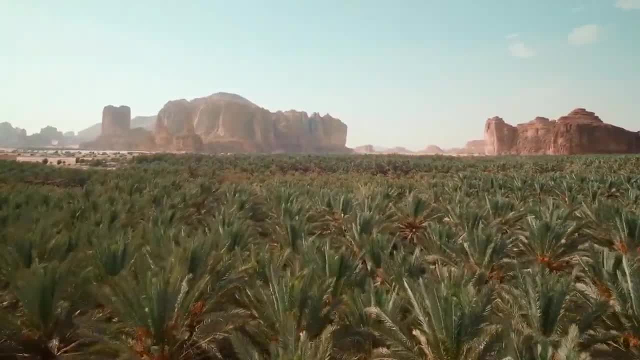 industries and technology will coexist in harmony with nature. Number 7. Green Riyadh. Green Riyadh is one of the major projects in Riyadh which started on March 19, 2019, under the guidance of King Salman bin Abdulaziz. 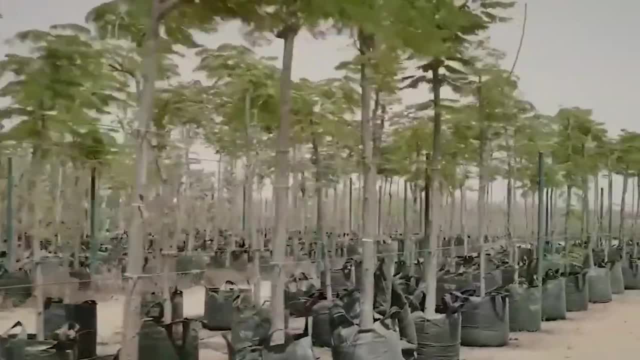 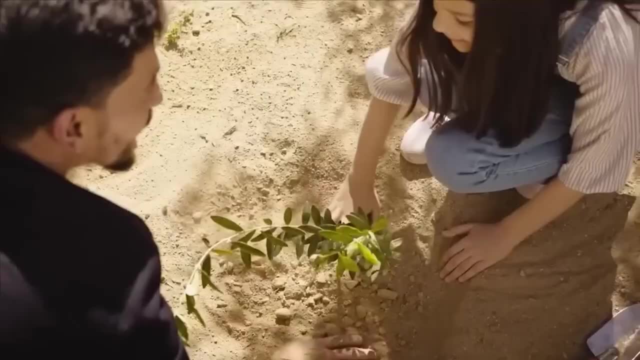 This project is a significant step towards achieving the goal of Vision 2030,, which aims to make Riyadh one of the world's top 100 most deliverable cities. The main objective of Green Riyadh is to increase the number of green spaces in the city. 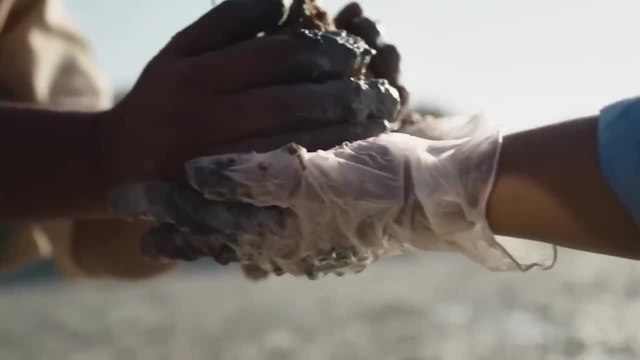 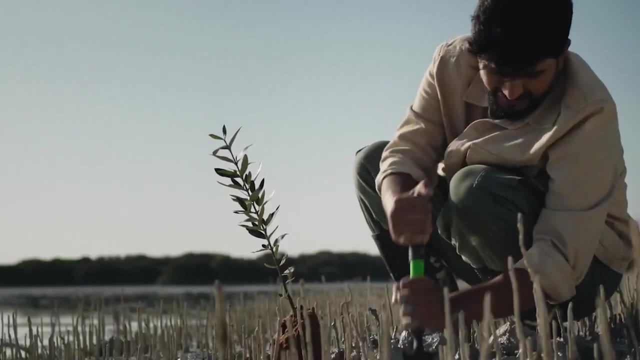 and enhance the overall quality of life for its residents. As part of this project, a whopping 7.5 million trees will be planted throughout Riyadh. These trees will be distributed across 3,300 nearby gardens, 43 parks, 9,000 mosques. 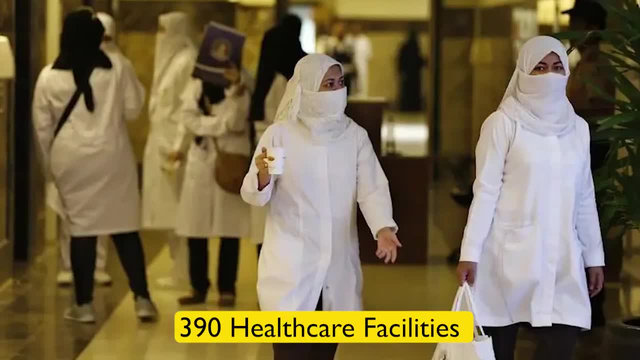 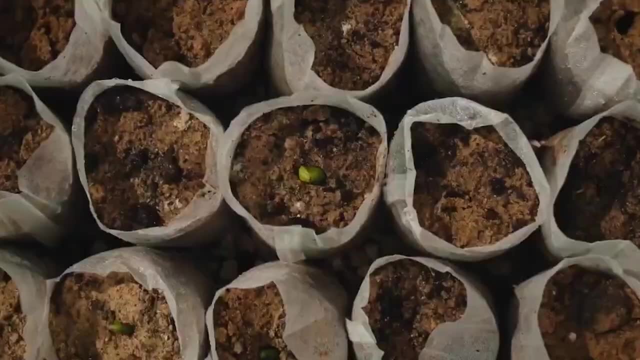 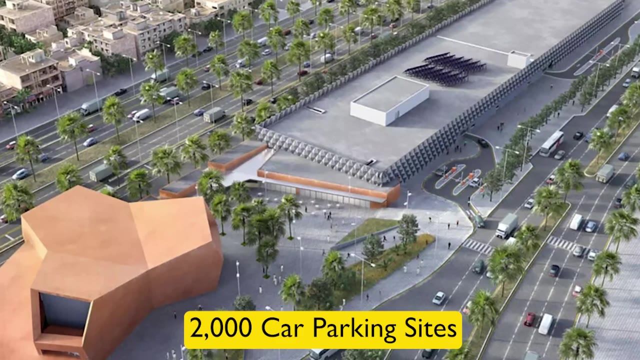 6,000 schools, 64 universities, 390 healthcare facilities and more than 1,600 public facilities. Additionally, trees will be planted along approximately 16,400 kilometers of streets and roads, as well as in 2,000 car parking sites, 1,100 kilometers of green belts and. 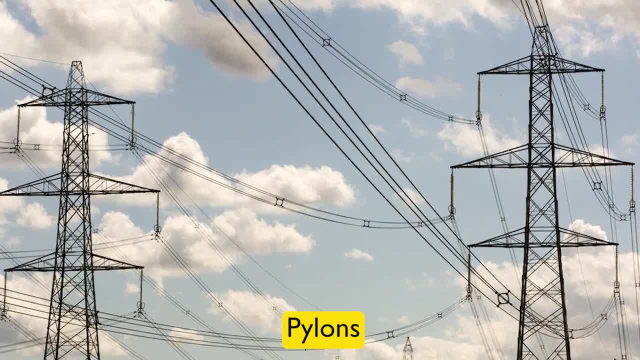 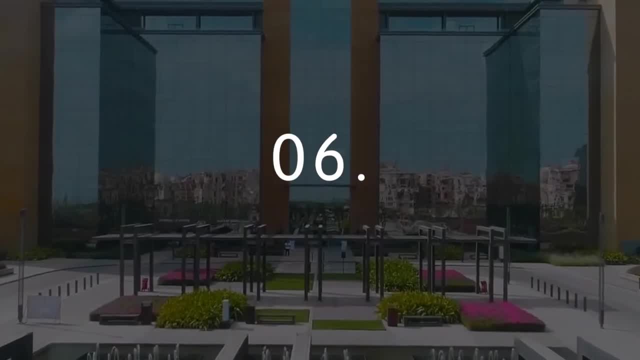 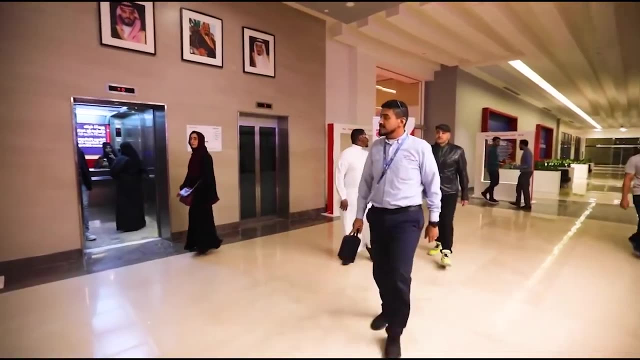 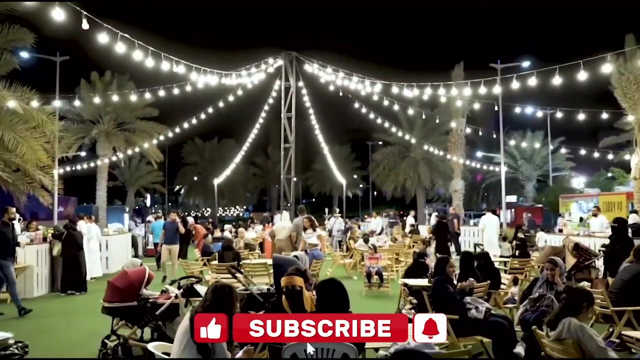 various other areas, including utility lights, phylons, oil pipelines, empty land plots and 272 kilometers of valleys. Number 6. King Abdullah Economic City. King Abdullah Economic City, or KAEC, is a large-scale development project situated along the Red Sea coast in Saudi Arabia. The aim is to create a modern metropolis. 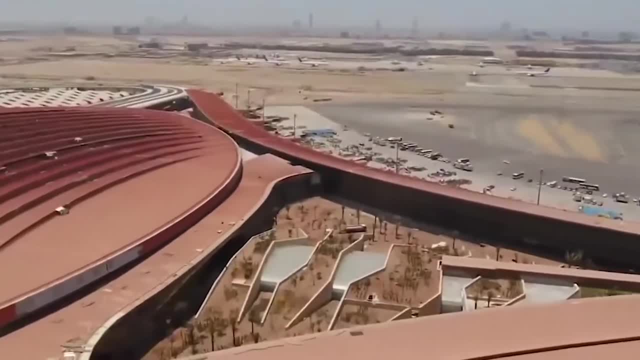 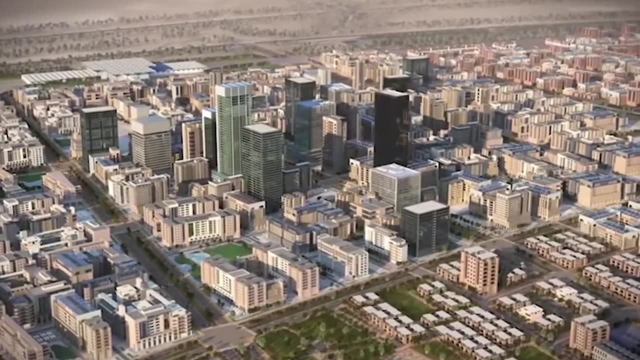 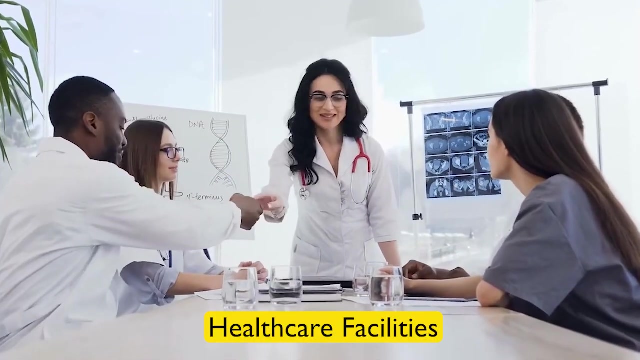 that offers its residents a high standard of living while substantially contributing to the economic advancement. The city will span over 173 square kilometers, incorporating essential amenities such as a world-class port, industrial zone, educational institutions, healthcare facilities, entertainment venues and residential areas. The projected population upon completion: 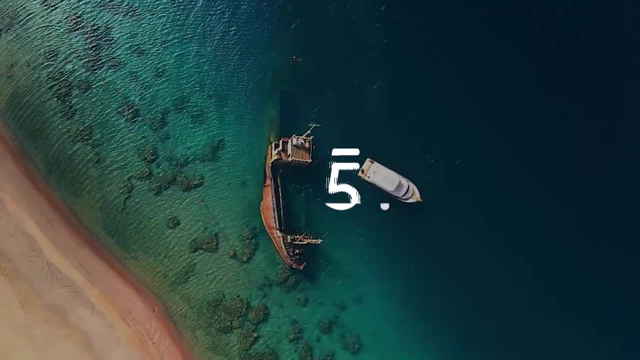 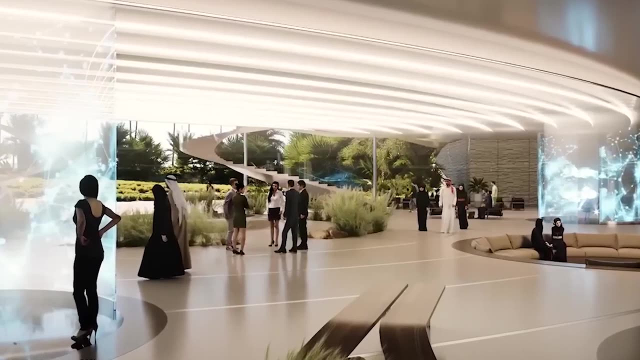 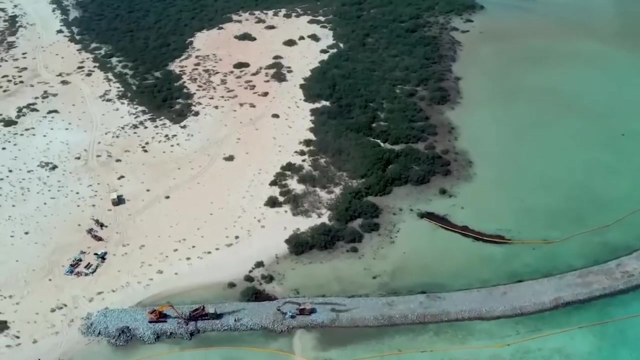 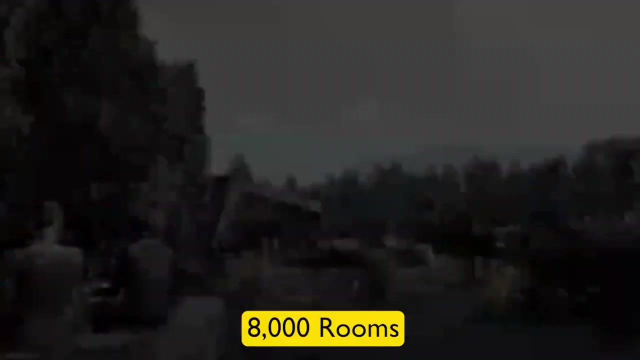 is estimated to reach 2 million people. Number 5. Red Sea Project. The Red Sea Project is a tourism development project located on the western coast of Saudi Arabia. It covers over 28,000 square kilometers and aims to attract visitors worldwide by offering luxury amenities and experiences. The project will include 50 hotels, over 8,000 rooms. various accommodations, recreational activities and cultural tours. The project also prioritizes environmental sustainability and aims to preserve the region's natural beauty. It is expected to create job opportunities and contribute significantly to the country's economic growth. Number 4. Jeddah Tower. 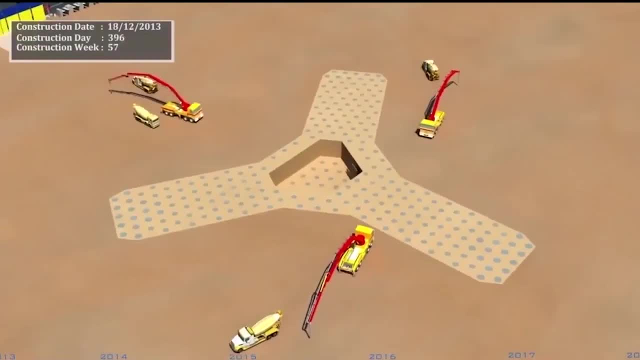 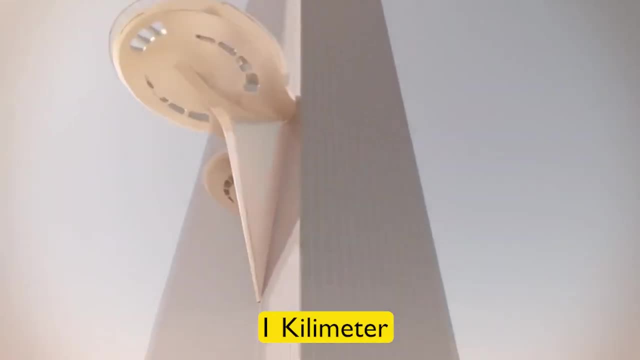 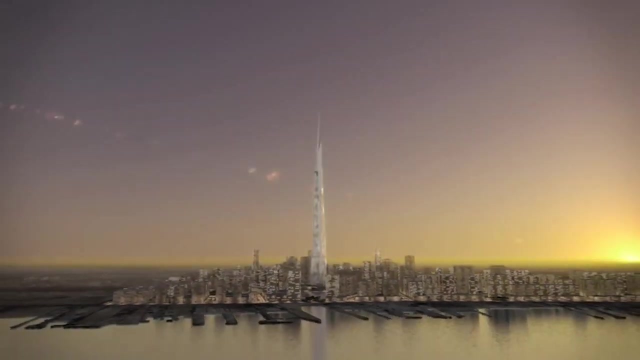 The Jeddah Tower currently under construction in Jeddah, Saudi Arabia, is an ambitious skyscraper set to become the tallest building in the world, reaching a height of over 1 kilometer. Its anticipated completion date is in 2023.. Inspired by Islamic architecture, the tower will 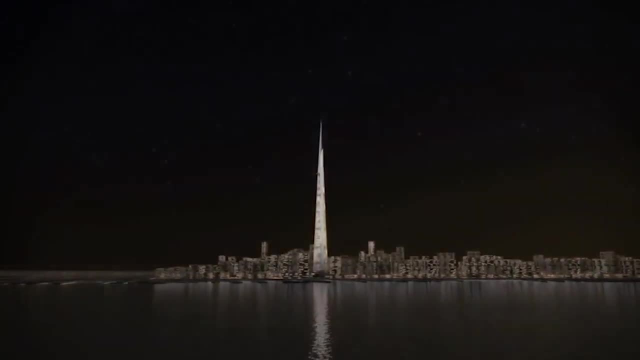 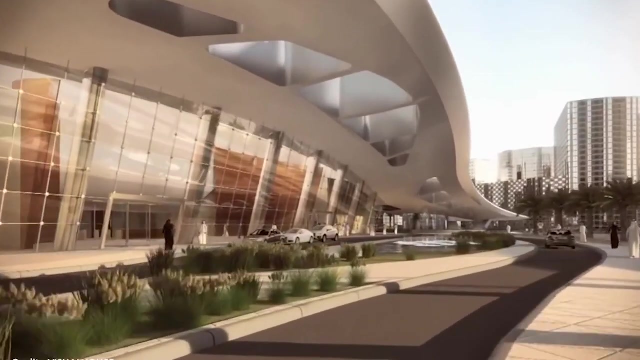 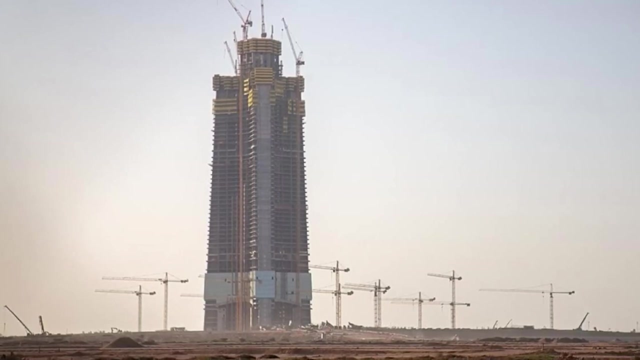 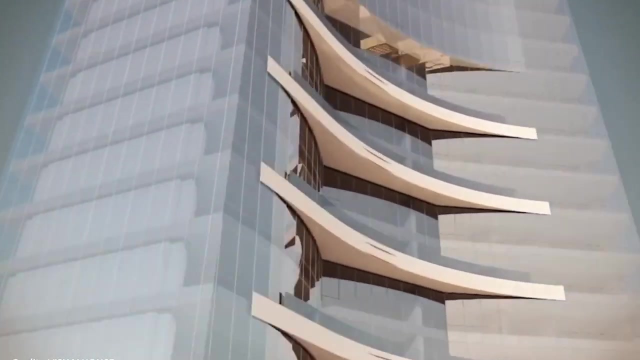 boast a distinctive design and will house luxury hotel accommodations, office spaces and residential facilities. It is poised to become a significant landmark in the city, symbolizing Saudi Arabia's economic growth and aspirations. However, the project has experienced delays due to financial and construction challenges, causing it to extend beyond the initial target completion year of 2021. 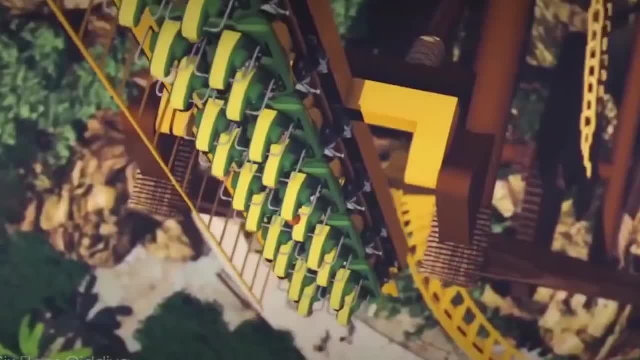 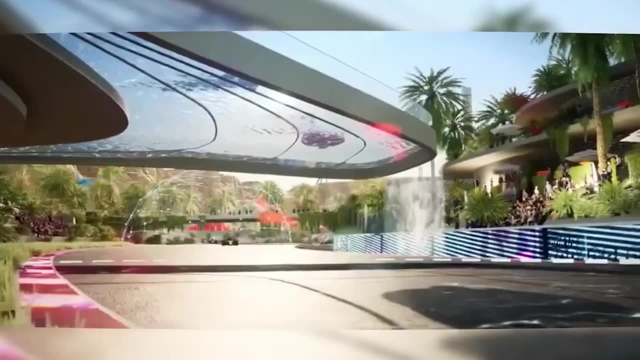 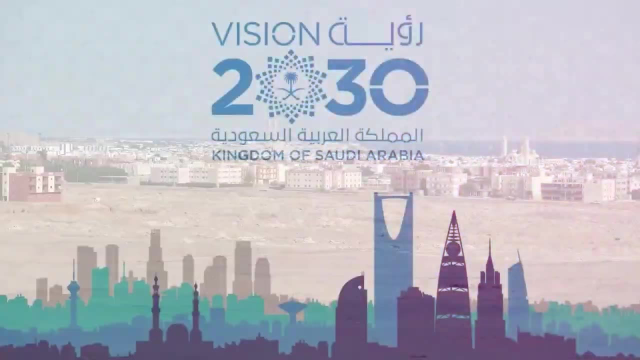 Number 3. Qadiyah Project. Qadiyah Project is poised to become an entertainment, sports and arts hub. It aims to revolutionize the concept of destination, tourism and recreation experiences by offering innovative and immersive activities on an unprecedented scale. This initiative aligns with Vision 2030's goal of enriching Saudi Arabia's 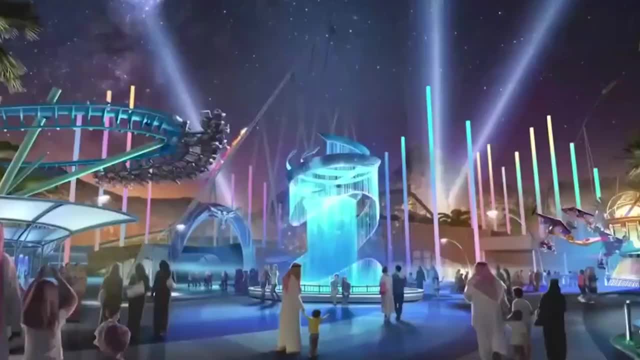 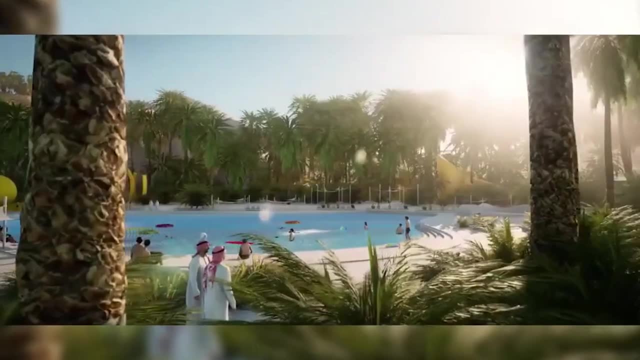 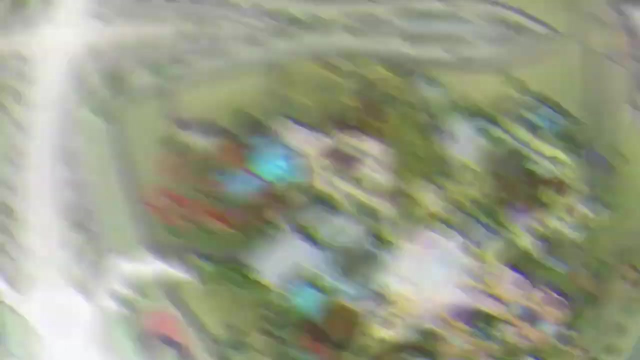 entertainment, culture and tourism offerings. The Qadiyah Project encompasses a diverse portfolio based on five core themes: parks and attractions, sports and wellness, motion and mobility, arts and culture. and nature and environment. The master plan has been meticulously designed to preserve and 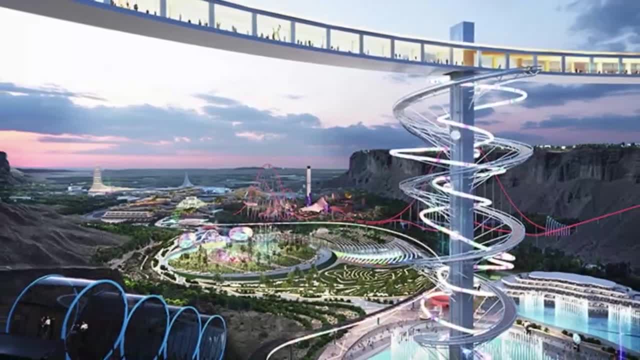 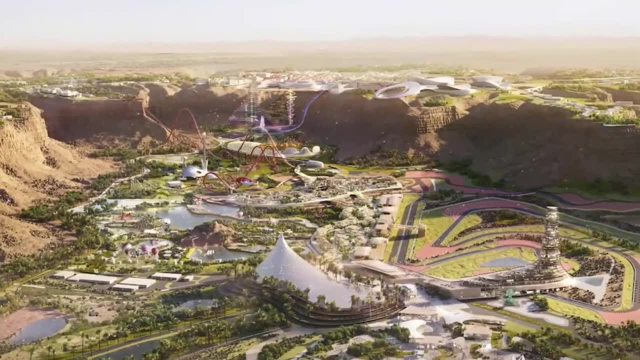 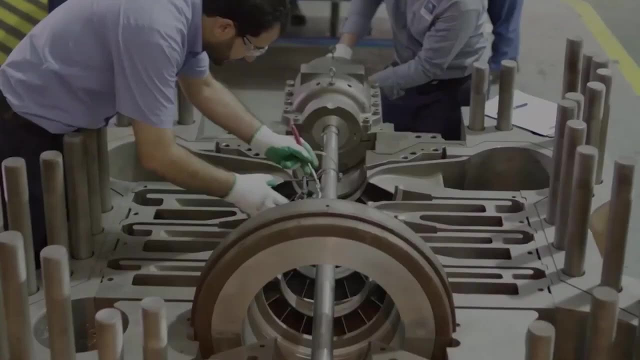 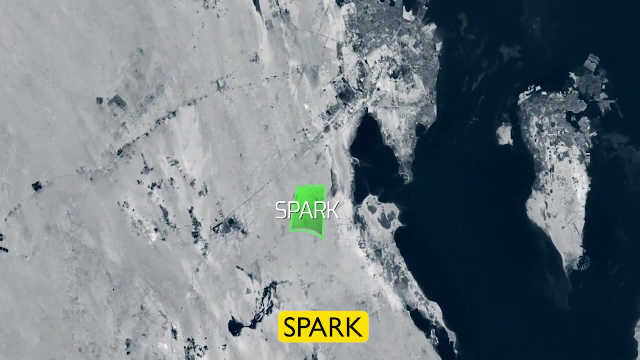 enhance the site's natural landscape. Key development nodes include the Resort Core, Qadiyah Village, Motion Zone, Eco Zone and Golf Community. Qadiyah represents a significant step towards realizing the country's cultural and recreational development vision Number 2. King Salman Energy Park. King Salman Energy Park, also known as SPARK, 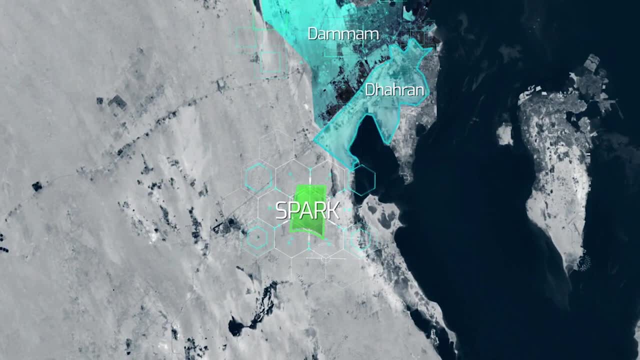 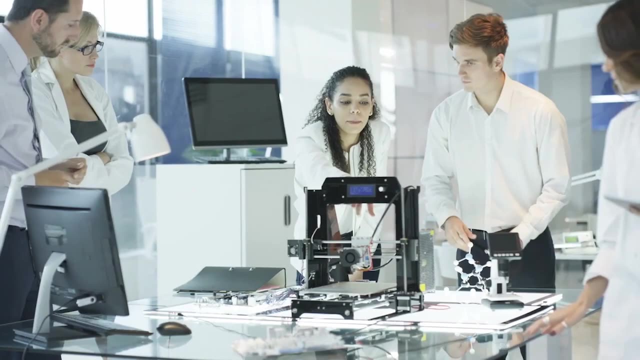 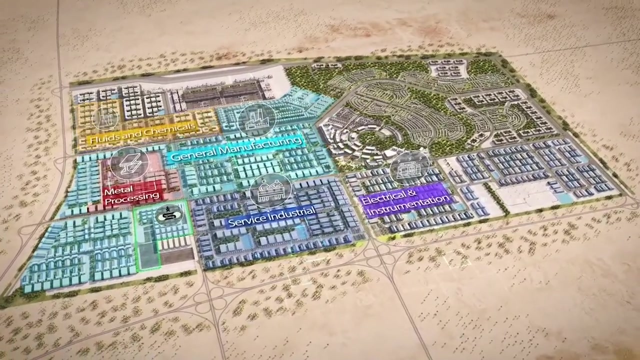 is an industrial park located in the eastern province of Saudi Arabia. It aims to attract local and international investors in the energy sector, while creating job opportunities for Saudi citizens. Spanning an area of 50 square kilometers, SPARK is a fully integrated industrial ecosystem. 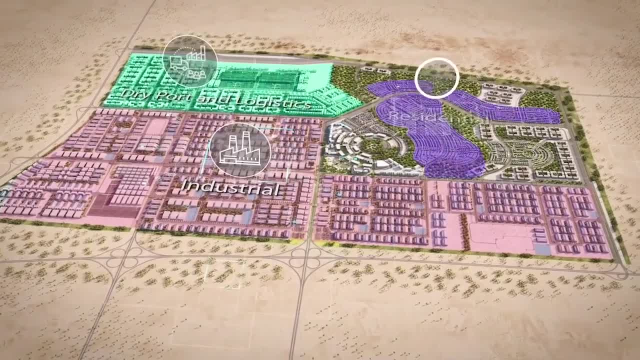 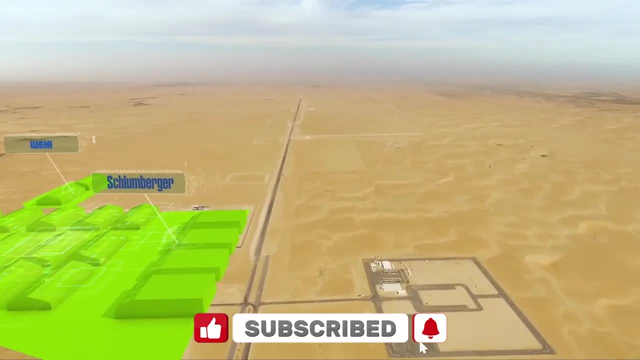 strategically positioned to become the region's primary gateway for the energy sector. As part of Vision 2030,, SPARK plays a crucial role in diversifying the kingdom's revenue streams and promoting a clean and sustainable region. Notably, it has achieved the remarkable distinction: 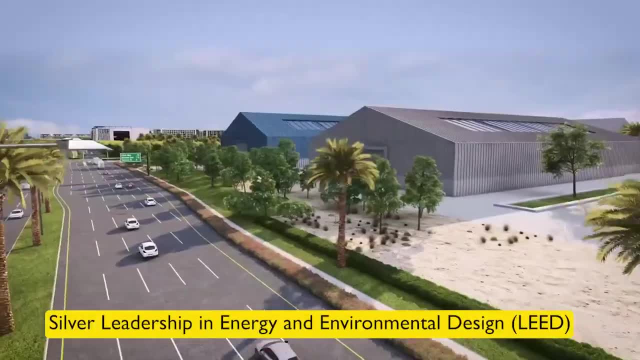 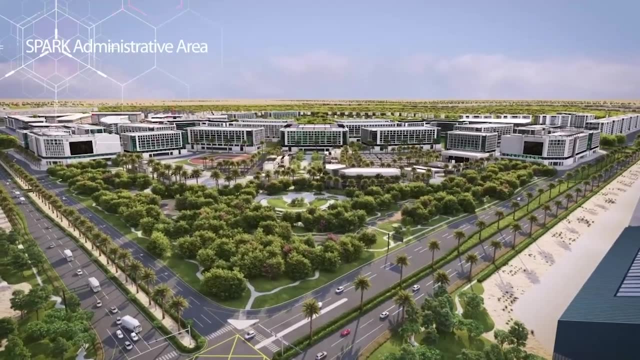 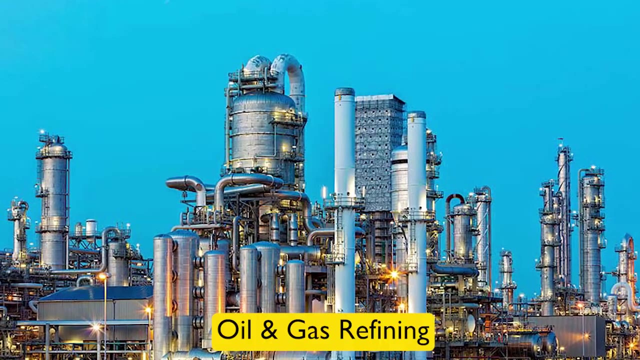 of being the world's first and only industrial city to receive a Silver Leadership in Energy and Environmental Design certification, SPARK offers state-of-the-art infrastructure built to international standards, catering to global investors in various industries, such as oil and gas refining, petrochemicals, energy and water production, and water treatment. 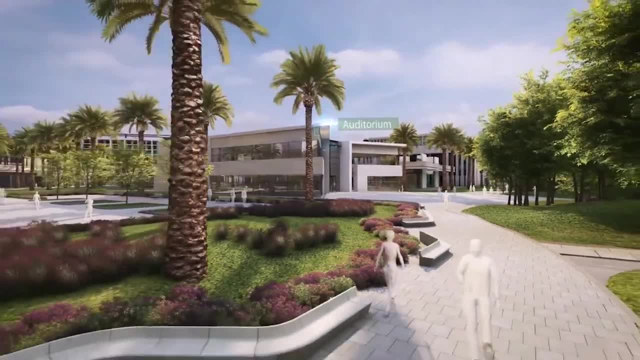 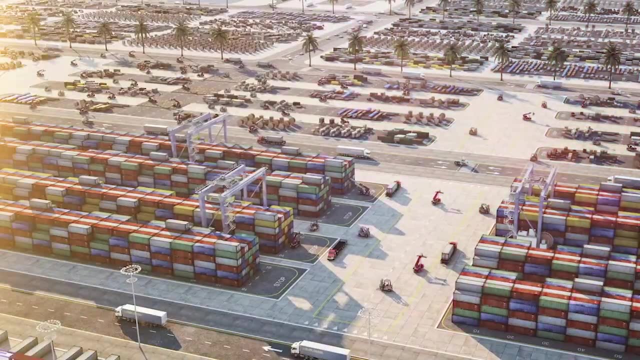 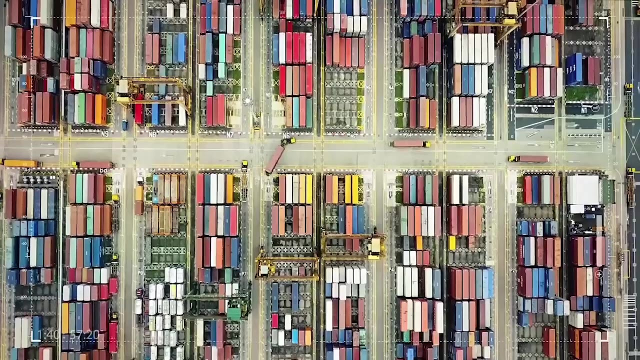 The construction of SPARK is planned in three phases covering an area of 14 square kilometers, and components of the first phase set to be completed by 2030.. The site also includes a dedicated three-square-kilometer logistics zone and dry port, further enhancing its capabilities. 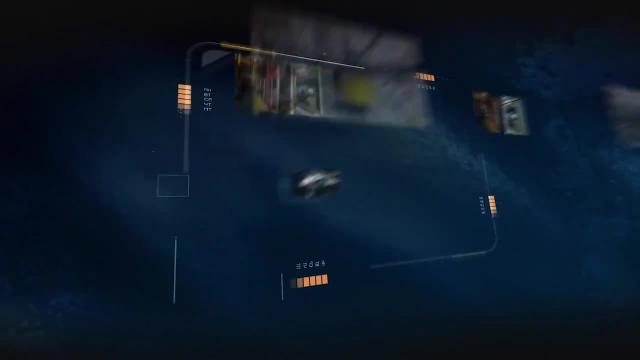 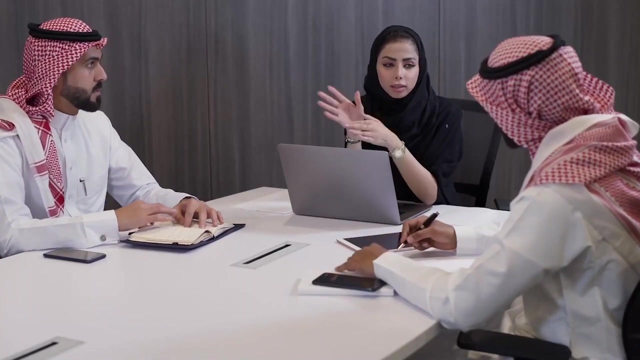 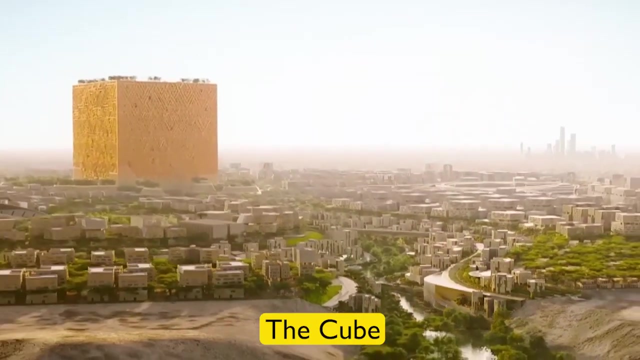 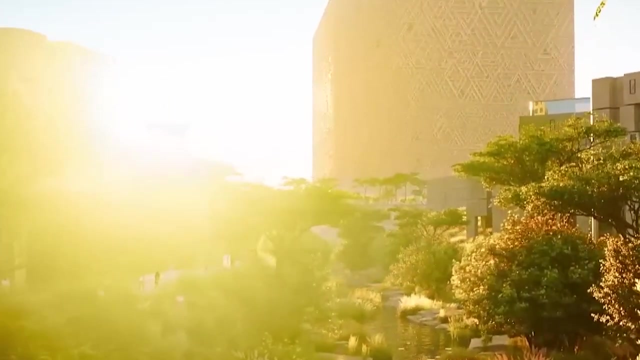 With its strategic location and comprehensive offerings, King Salman Energy Park is poised to be a key driver of economic growth, investment and sustainable development in the energy sector. Number 1. Muqab Muqab, meaning the cube, is an ambitious project in Saudi Arabia. It aims to construct a massive cube-shaped skyscraper.